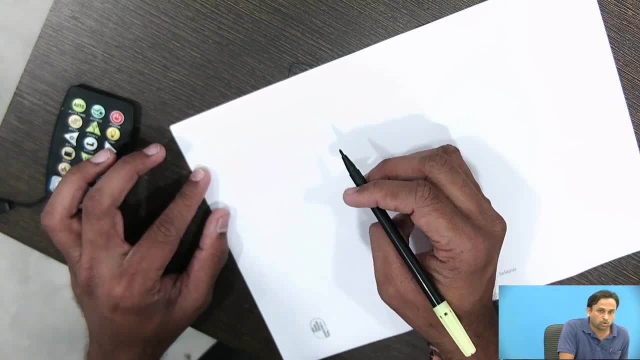 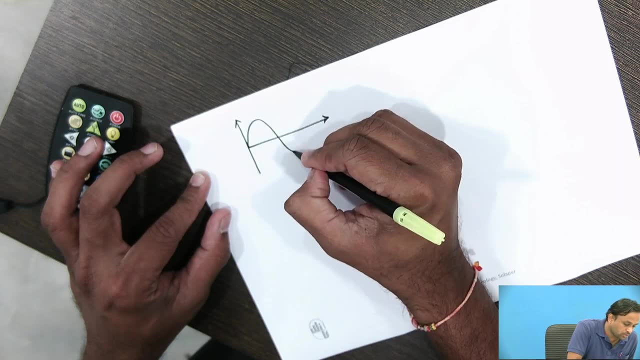 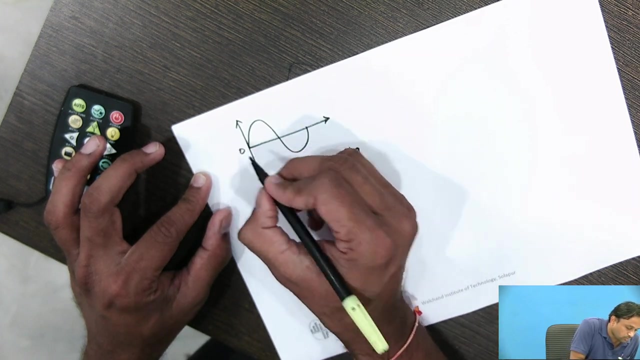 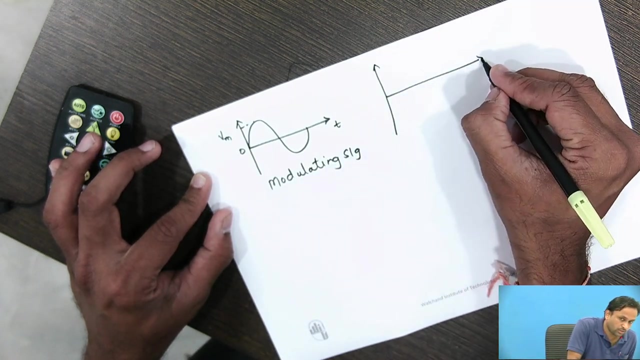 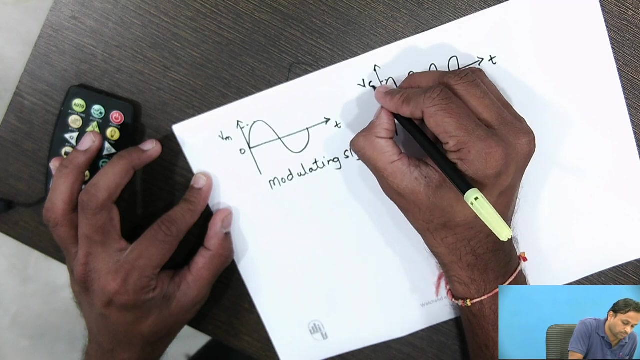 Okay now, as we know, for modulation we required two signals. which is there? okay, so this is modulating signal. so this is an amplitude of an modulating signal. this is steam. so one more signal, that is carrier signal, whose amplitude is- we see whose amplitude is VC. 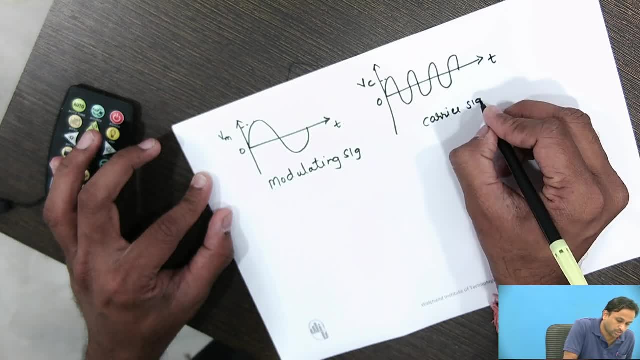 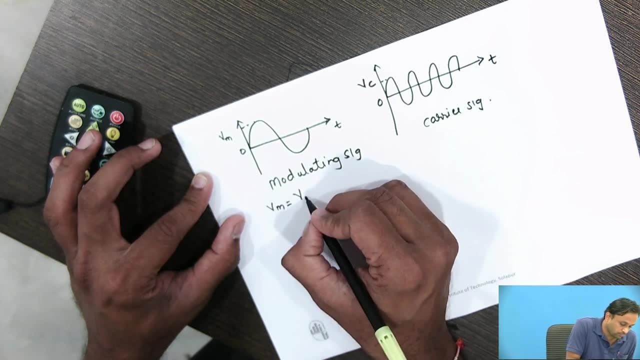 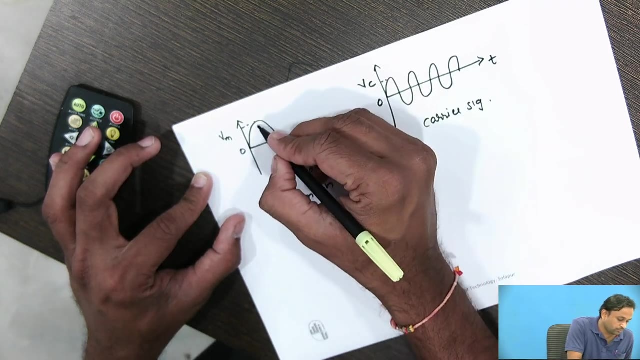 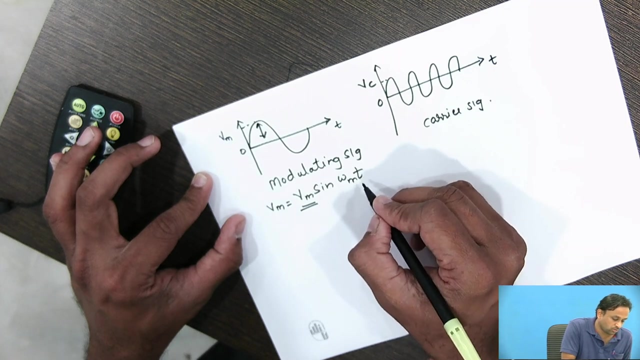 here. so this is carrier signal. so if you define the equation for an modulating signal, so it will be VM, VM sine Omega M of t. this is amplitude of an, the modulating signal, this will be an frequency and phase, and frequencies are kept constant. so that's why we are not going. 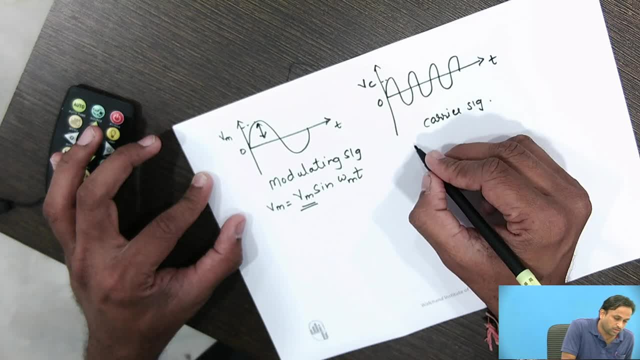 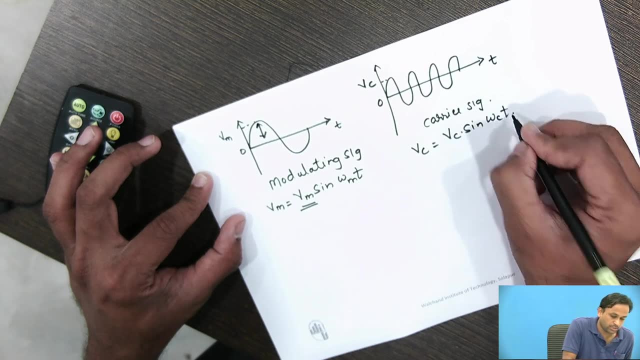 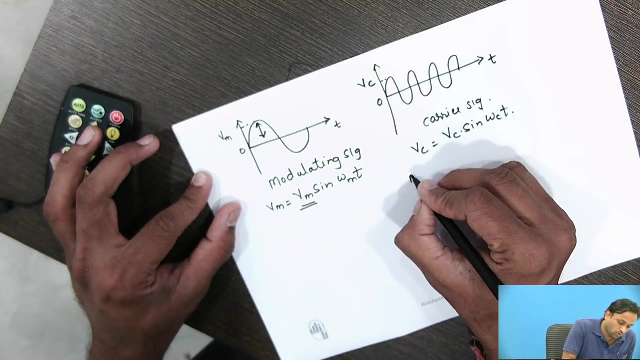 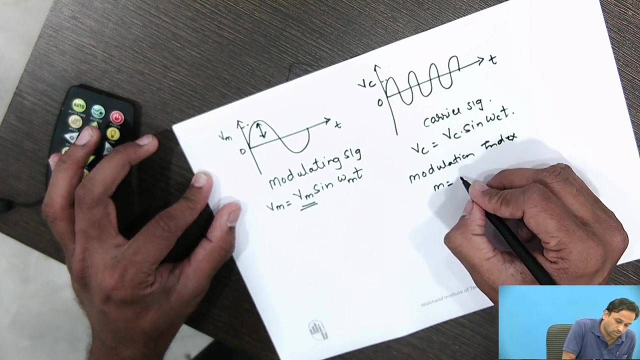 to take this into this equation here. similarly, for carrier equation c will be vc by vc, sine omega, c, t. so before starting to the equation, so we have to understand what do you mean by modulation index here. so modulation index is defined, that is, vm is equals to vm by vc. that 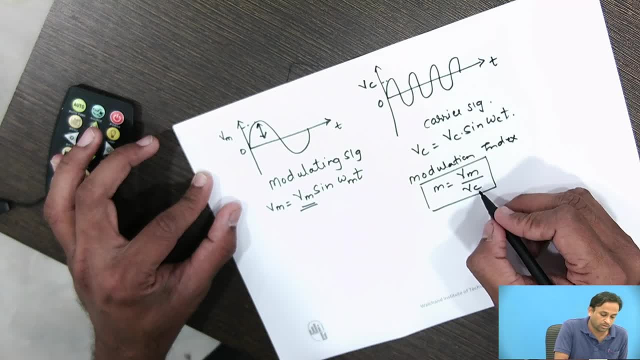 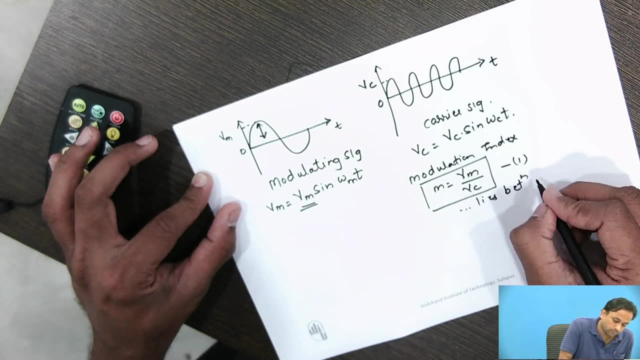 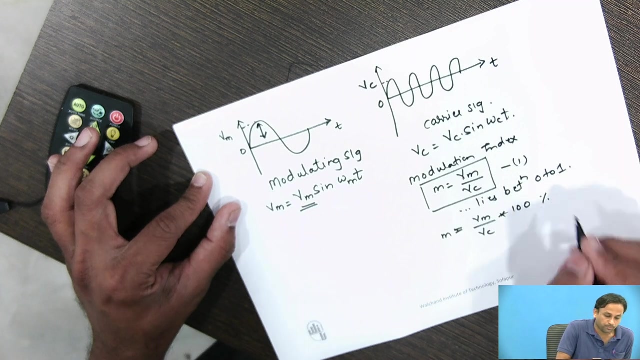 is amplitude of an modulating signal, to the amplitude of an, the carrier signal here. okay so, which lies between 0 to 1. okay, if you have to calculate in percentage, then we have to multiply by 100, okay, okay, so vm by vc into 100 here. so we will get into the percentage. okay, so now we will have the. 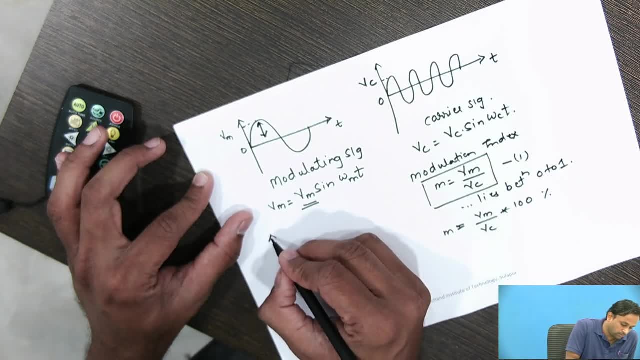 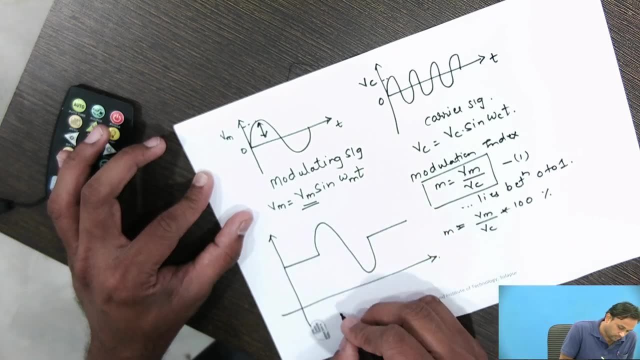 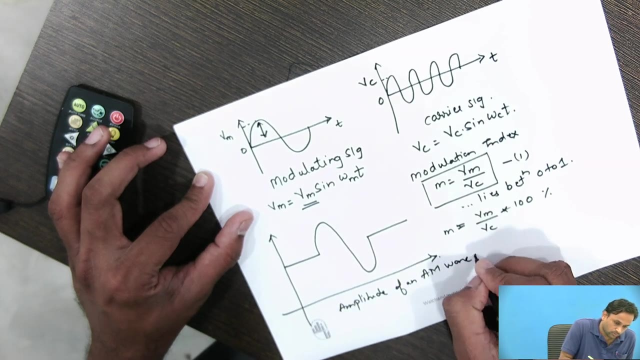 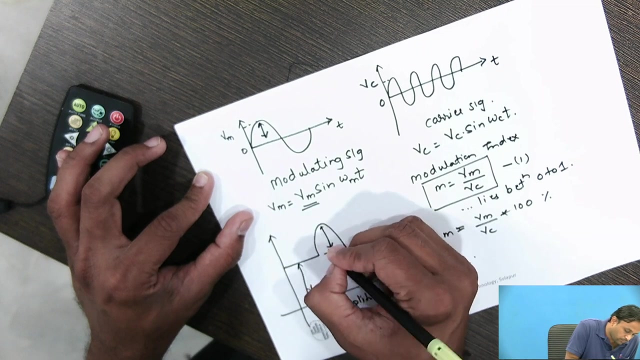 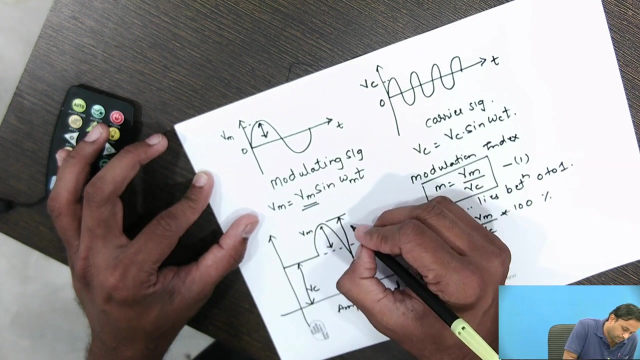 amplitude of an am wave. so we will derive the equation. so for that we required one diagram. okay, so this is an amplitude of an am wave. okay, so this is vc, this will be vm. okay, and this total will be a. that is total amplitude of an vm plus vc. okay, and 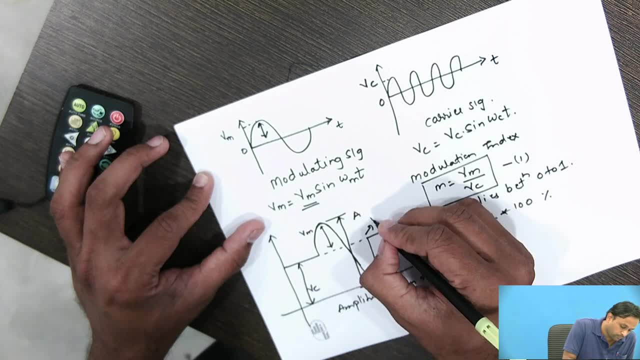 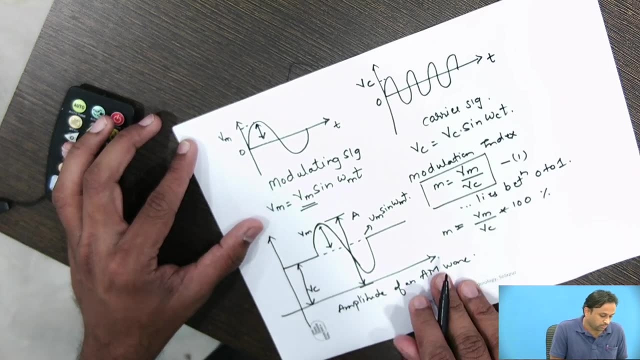 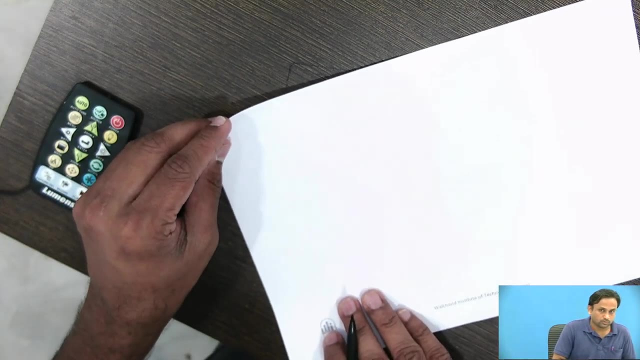 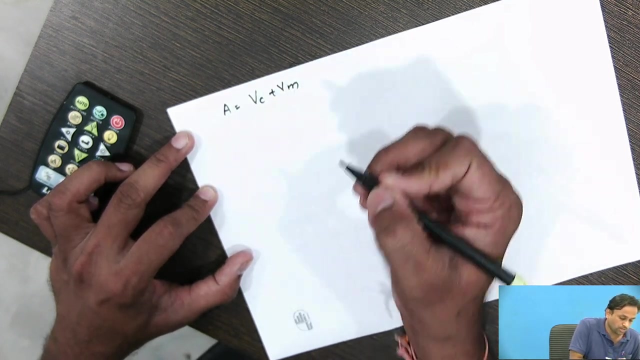 the equation for this modulating signal will be vm sine omega m of t here. okay, so first let us derive the total amplitude of an am wave. total amplitude of an am wave. total amplitude of an am wave wave. total amplitude of an am wave. okay, so we have a equals to vc plus vm. vc plus vm. 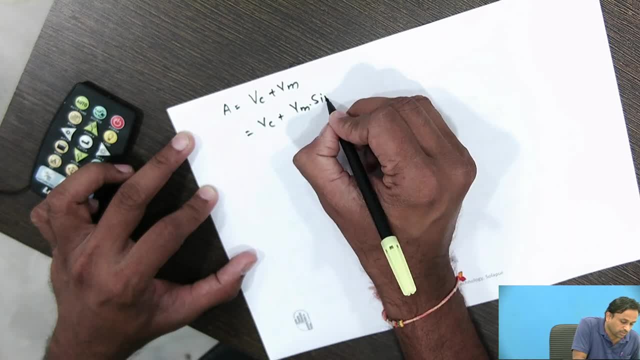 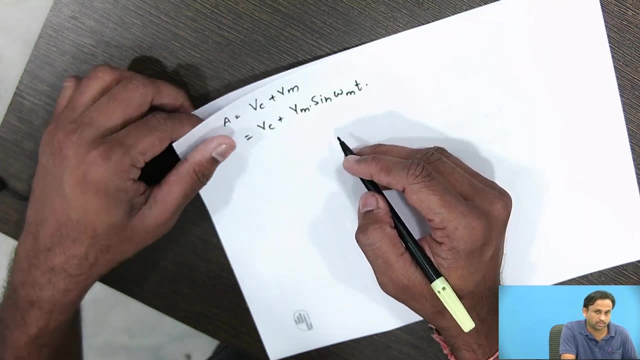 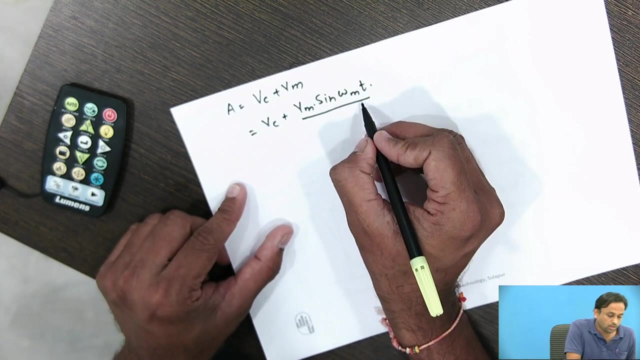 so vc is equals to vm sine omega m of t, because we are going to change with respect to amplitude of an modulating signal. that's why we have to take total signal, that is, vm sine omega m of t, instantaneous value of n, the modulating signal. here, therefore, we are going to take common vc. 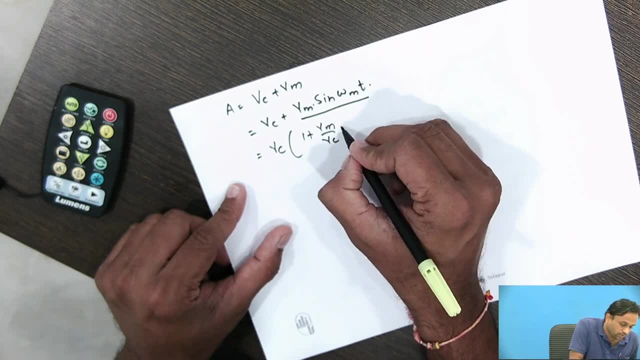 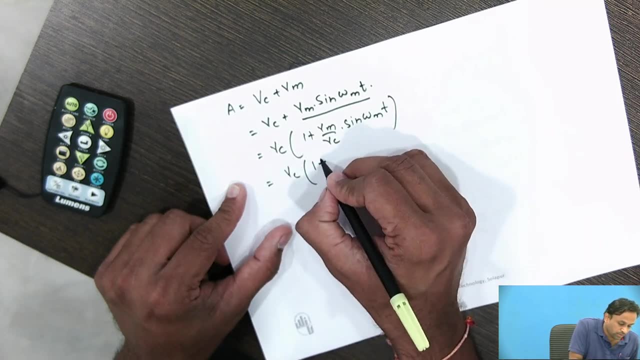 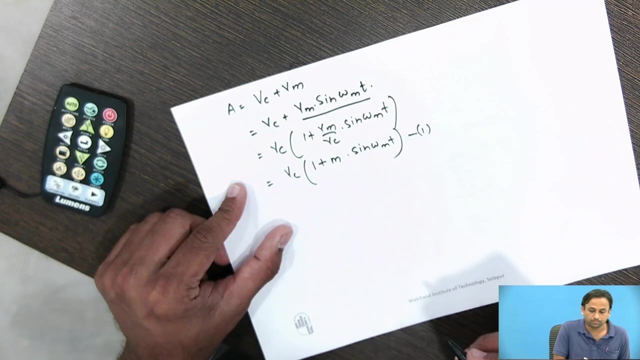 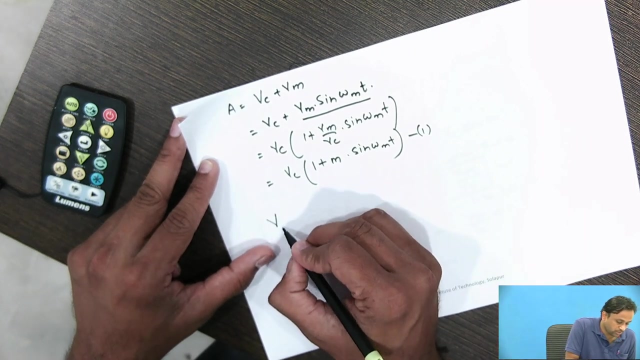 1 plus vm by vc sine omega m of t. so which will be vc? substituting the value of an m, that is m, is vm by vc, here sine omega m of t. so this is equation, you one. okay. so now we'll have the total instantaneous voltage, that is, total instantaneous voltage of an. 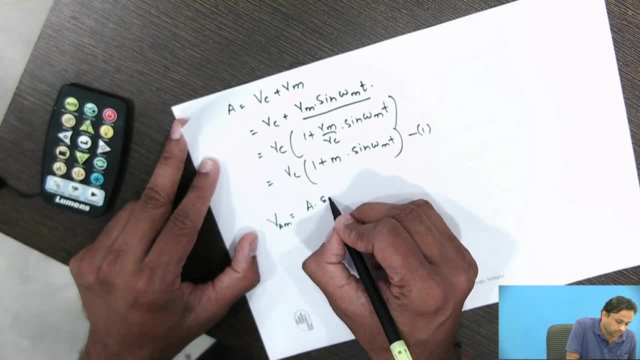 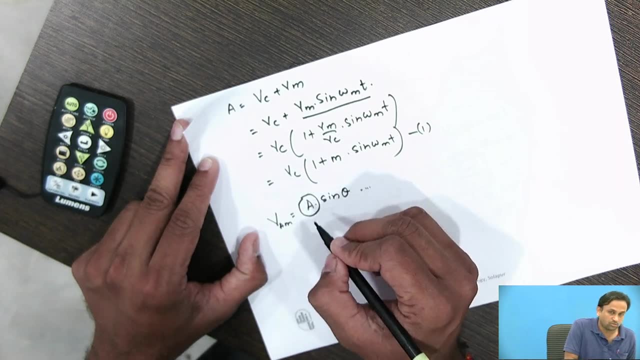 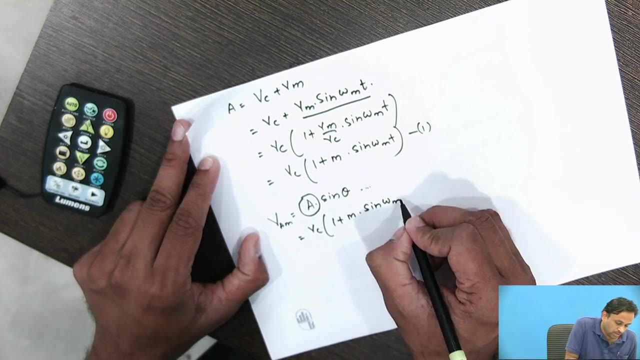 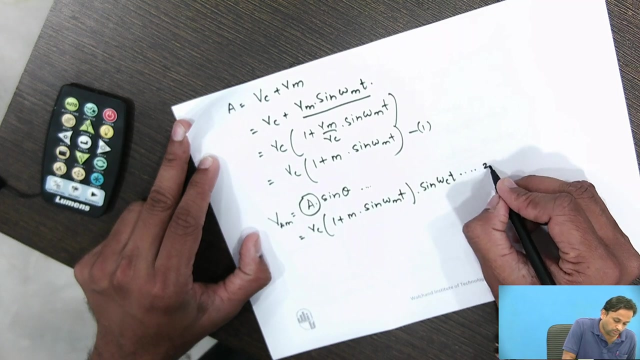 am. so for that we has to be a sine theta instantaneous voltage here. okay, so now substituting the value of an a into this equation, so you will be having vc 1 plus m, sine omega m of t into sine omega ct. okay, okay, so this is also one equation of an am signal. okay, so now by technometrical relations like 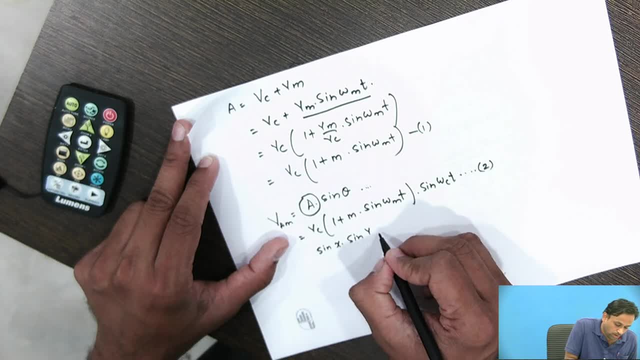 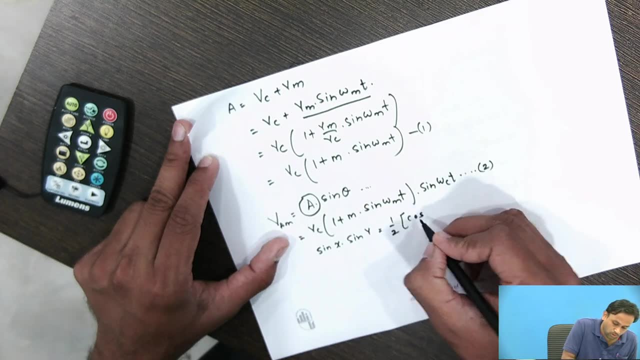 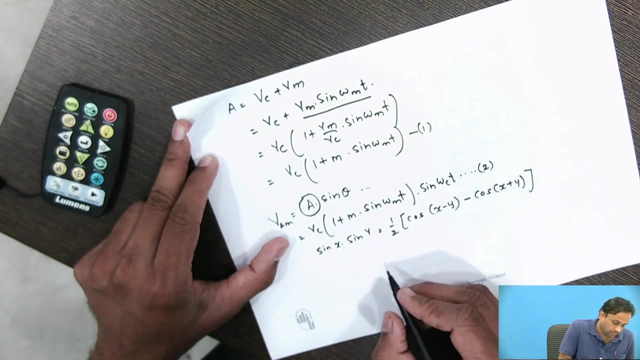 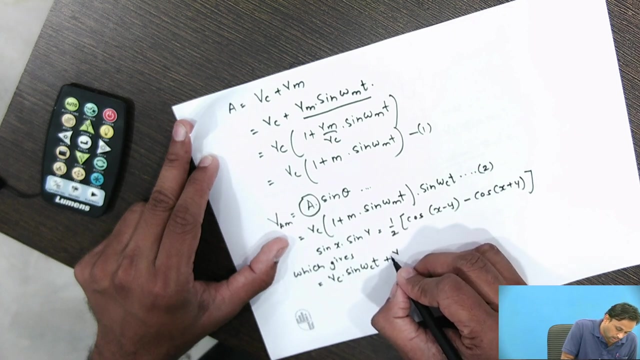 sine x into sine y, so we have to solve sine x and sine y, so which is half cos x minus y, minus cos x plus y. okay, so this is the relation. so which gives, which gives, that is vc sine omega ct plus v m, vc by 2 cos omega c minus cos m of t. 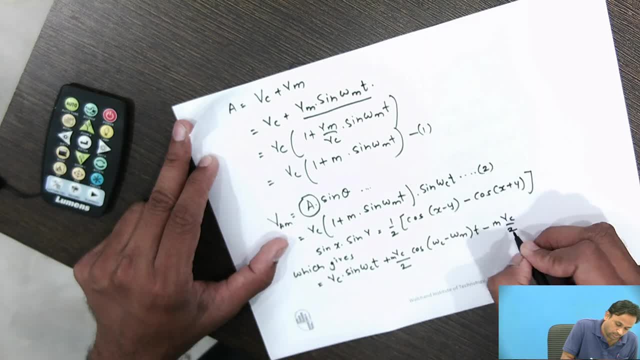 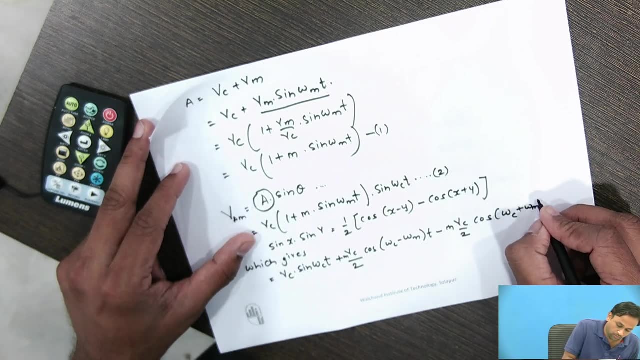 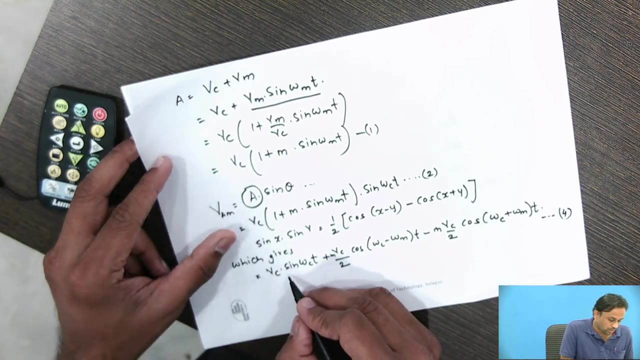 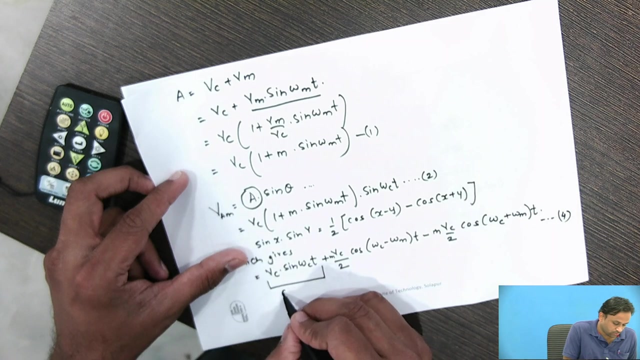 minus m vc by 2 cos omega c plus m of t. okay, so this is the final equation for an amplitude of an, this modulation, amplitude modulation. so now from this what we can analyze? that this is the same equation which is there for carrier signal. okay, so this is. 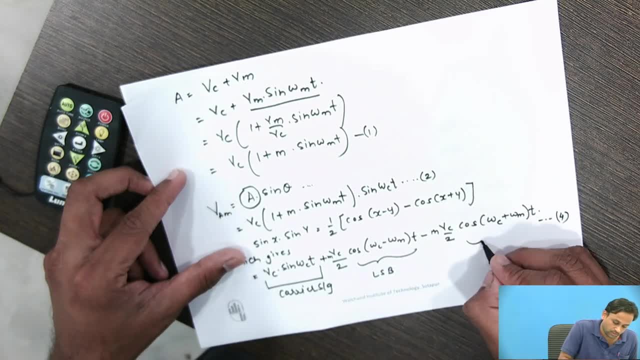 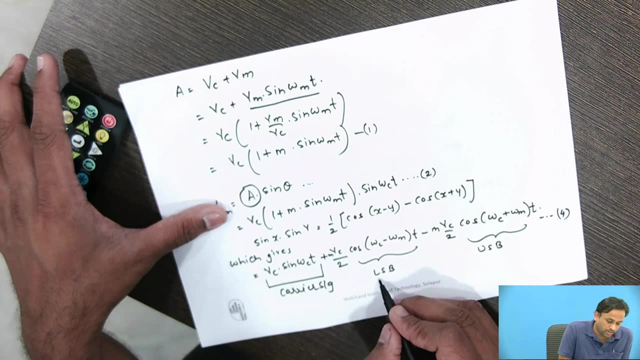 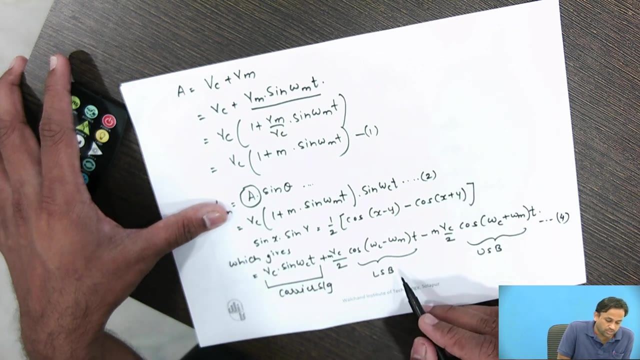 lsb, that is lower sideband and this is usb, which is called as an upper sideband here. okay, and the amplitude of an lsb and usb are m vc by 2 and here m vc by 2 here and the information contained in the amplitude modulation, this sidebands will be the same here with carrier. 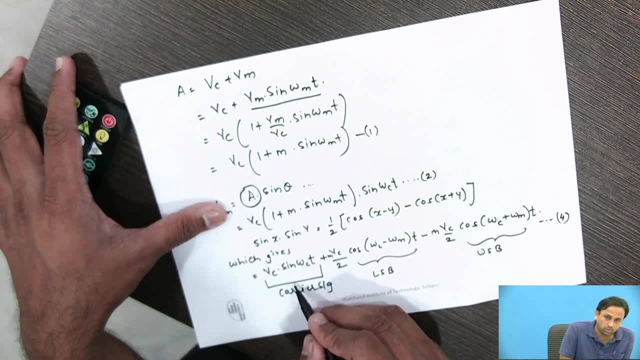 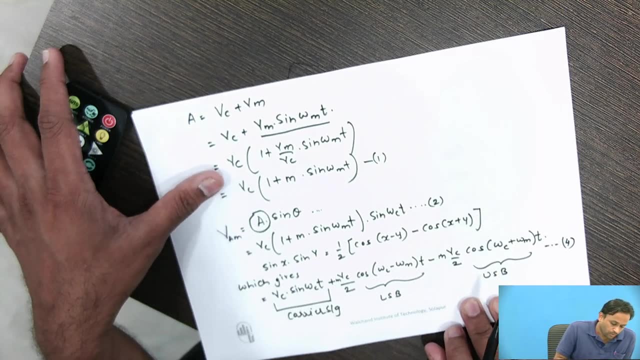 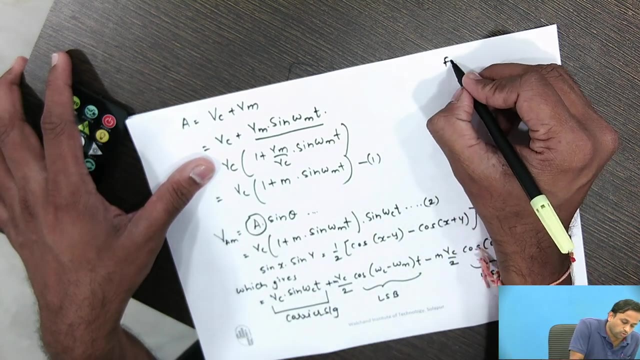 signal here, okay, so which gives three components in amplitude modulated equation, that is, carrier signal, lsb and usb here okay. so now we will see how to plot and amplitude modulation signal in frequency domain. so for frequency domain, if you have to analyze this signal, we have to make use. 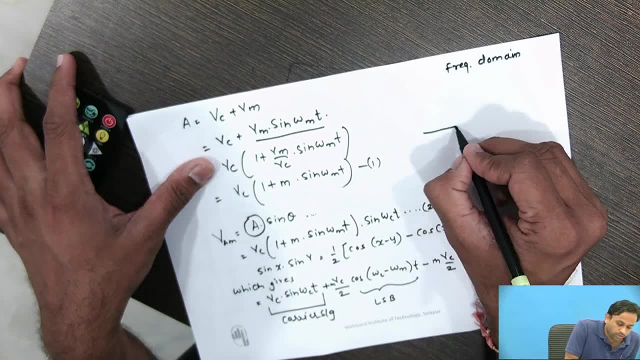 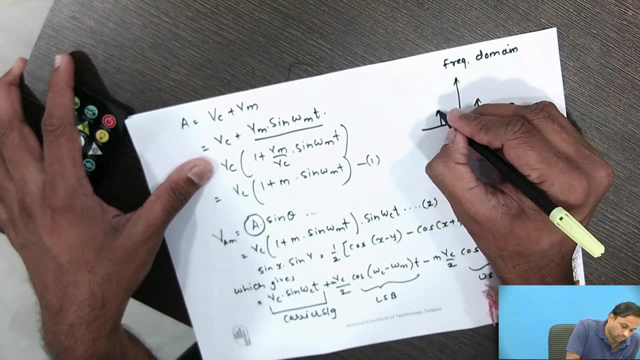 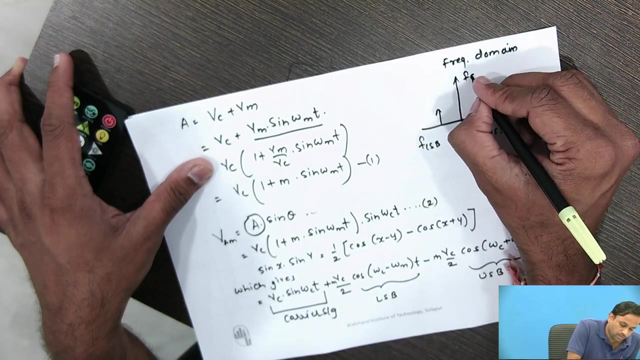 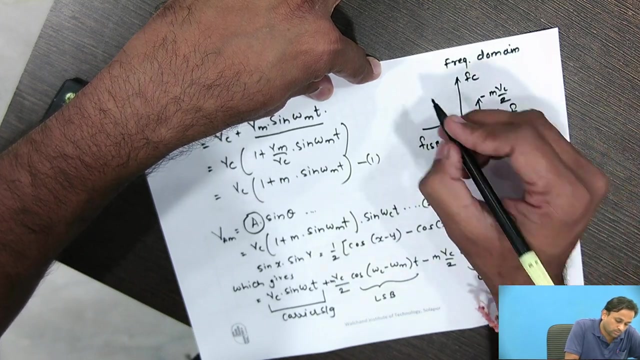 of an spectrum analyzer here. so in that we are going to see with respect to frequency, okay. so there, you will look like the signal in this manner here. so this will be f usb, this will be f lsb, this will be an fc here, okay, and this will be amplitude of an. the sidebands m. 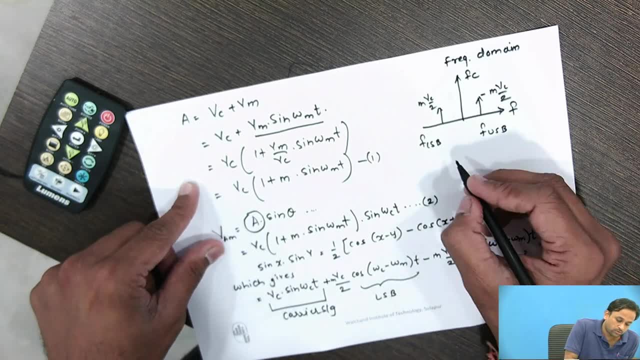 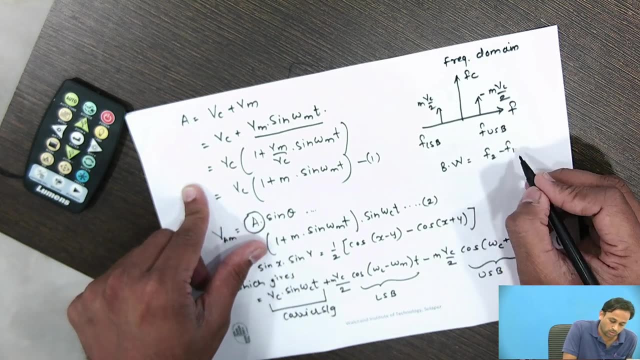 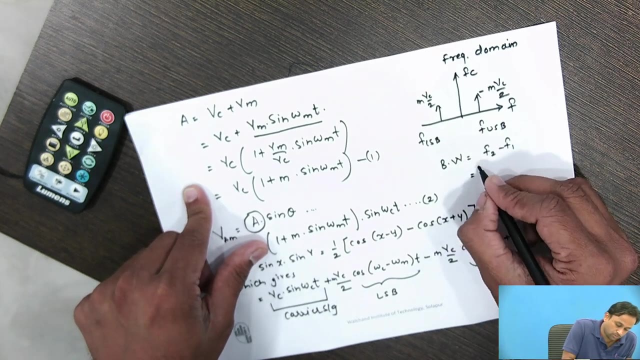 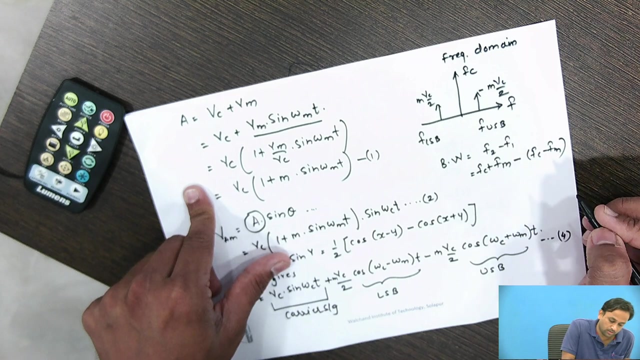 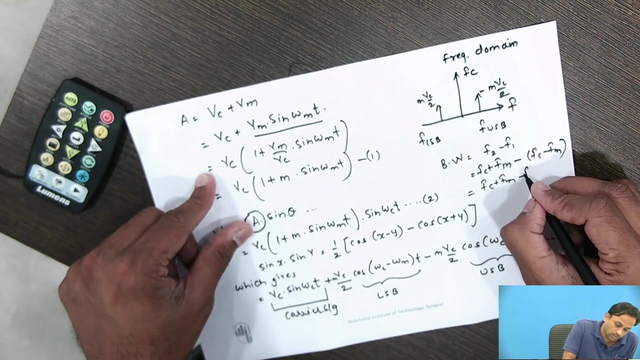 vc by 2. okay, so, if you calculate the bandwidth, so which is f2 minus f1, that is upper cutoff frequency minus lower cutoff frequency. upper cutoff frequency means usb, that is upper sideband, that is omega c plus omega m, so which we can write fc plus fm minus. you can write fc minus fm here. okay, so from this fc plus fm minus, fc plus fm, so